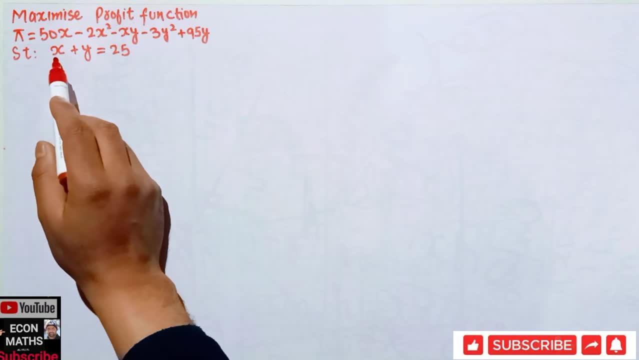 goods produced and subject to the constraint, that is, x plus y is equal to 25.. We have to maximize this profit function with respect to the constraint given, So we will use the Lagrange's function method. That is first of all we know from the previous videos. this is called: 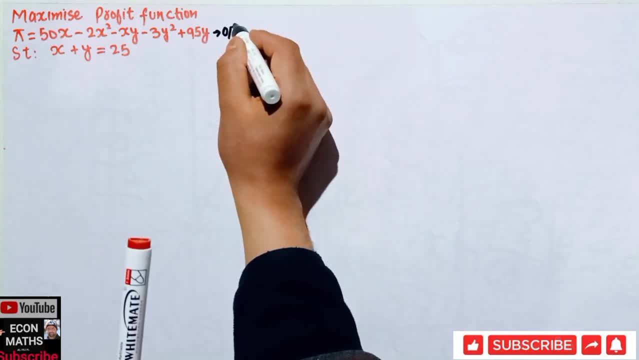 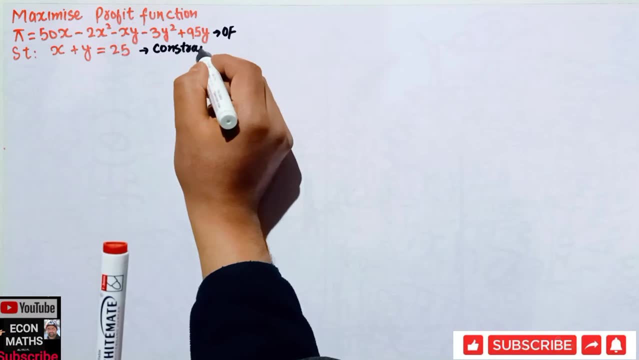 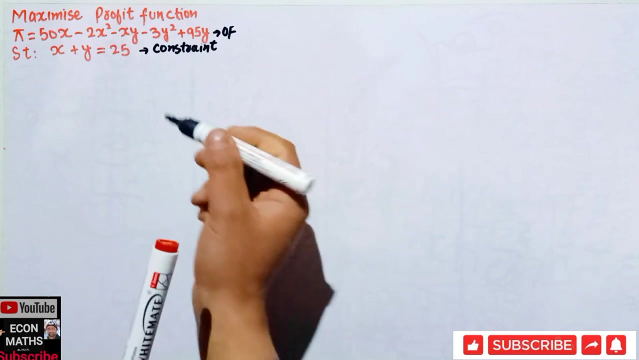 objective function, This is our objective function and this is called the constraint part. So I will write: this: is this is this is a corner strand. First of all, the first step in solving this question is: first, we set this corner strand equal to zero. So we set this corner strand equal to zero. So I will write set: 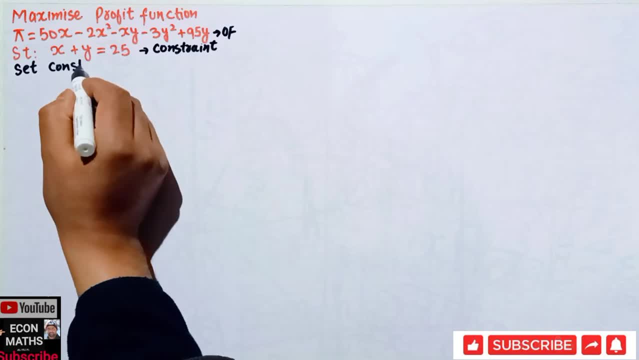 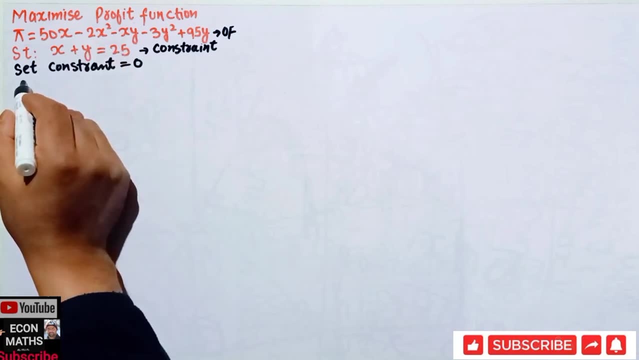 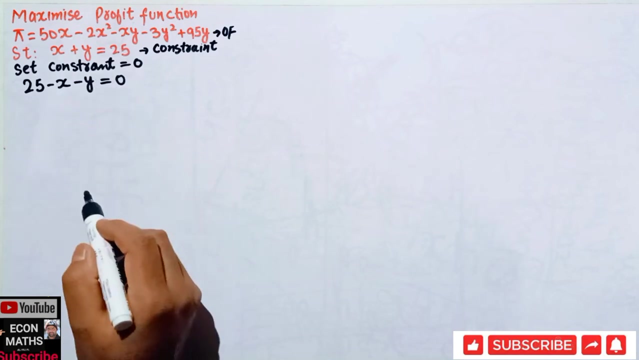 corner strand. corner strand equal to zero. That implies this whole thing will be equal to zero. I will write it as 25 minus x minus y is equal to zero. Second step is to multiply this very corner strand by lambda. So we will multiply this very corner strand. 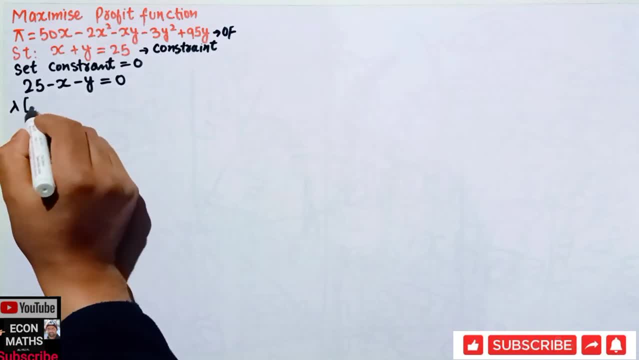 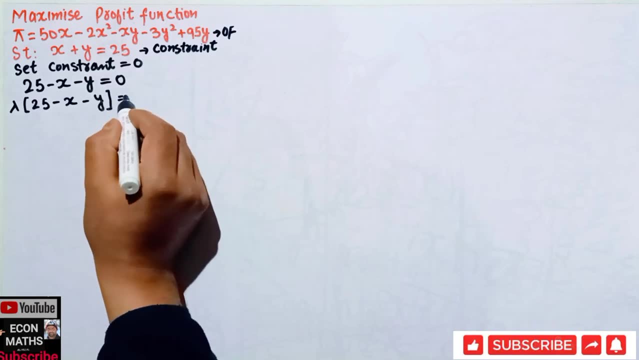 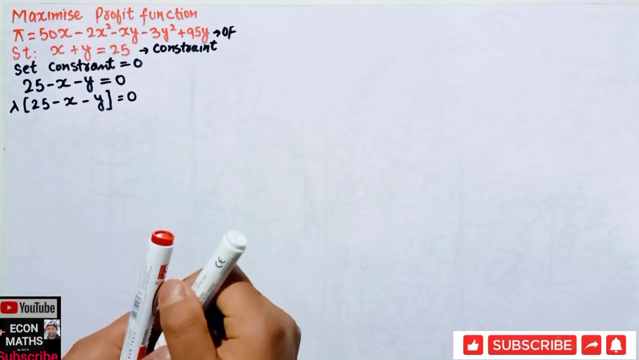 by lambda. So this will become lambda times 25 minus x minus y is equal to zero. Now we have to form the Lagrange's function. That is, the Lagrange's function is formed by adding the objective function function with the resulting constraint function. so our lagrangian function is that is i will. 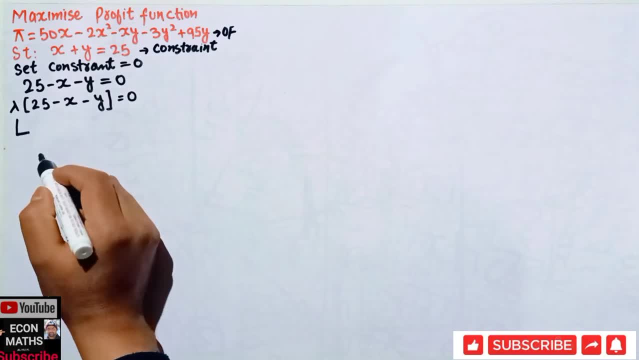 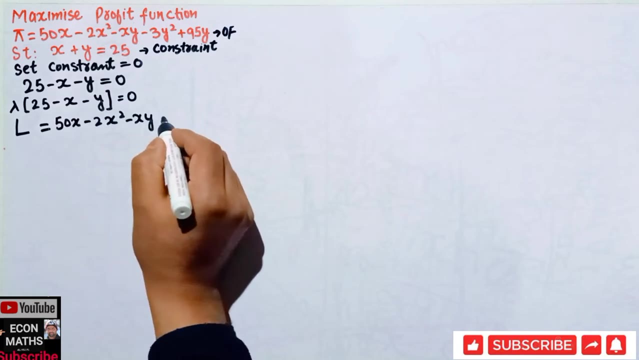 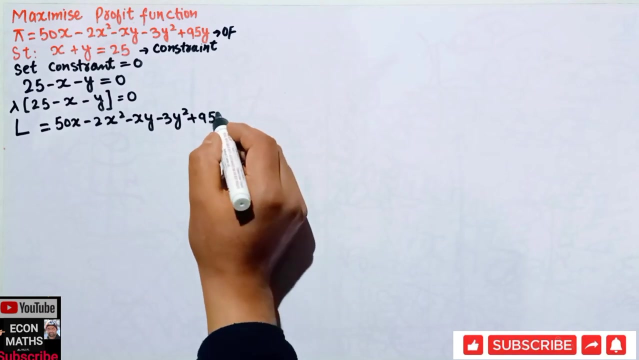 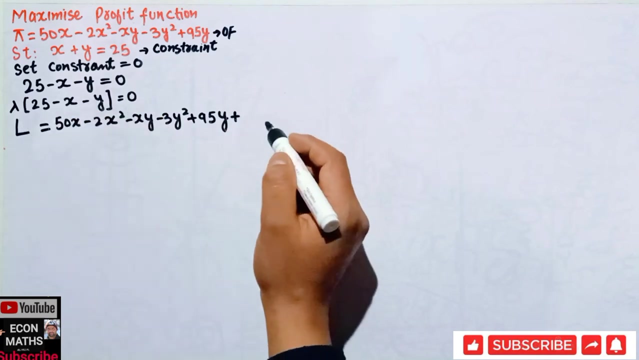 denote it by l. that means our lagrangian function is equal to the objective function, which is this very part, that is, 50 x minus 2 x square minus x y minus 3 y square plus 95 y. and we will add it the this very resulting constant, that is lambda times 25 minus x minus y. 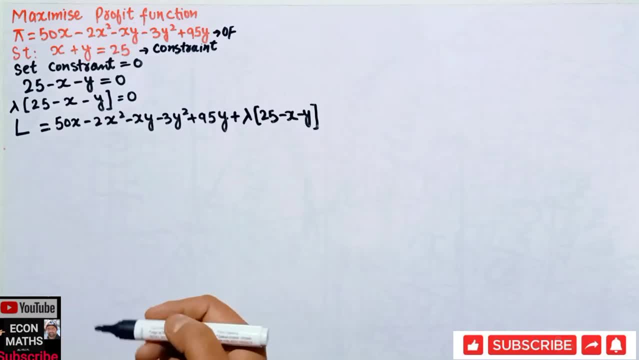 okay, now the next step in solving uh, this very lagrangian function, is, that is uh, to find the optimal values of x, y and lambda. we will partially differentiate this very lagrangian lagrangian function with respect to firstly by the x, then by z- sorry, y- and by the lambda. 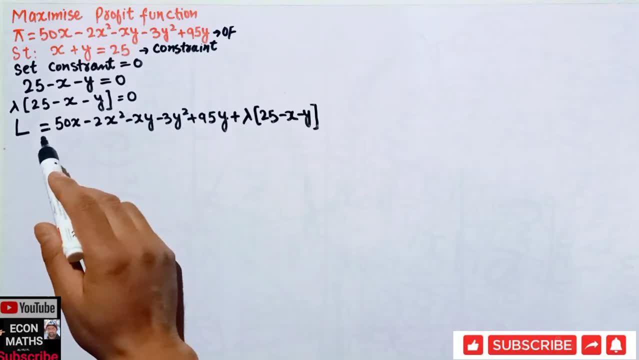 subsequently. so first we will partially differentiate this lagrangian function with respect to x and set it equal to 0, that is. i will denote l subscript. x means partially differentiating this lagrangian function with respect to x, so this will become the derivative of x. in this 50, x is 1, so this will become here 50.. 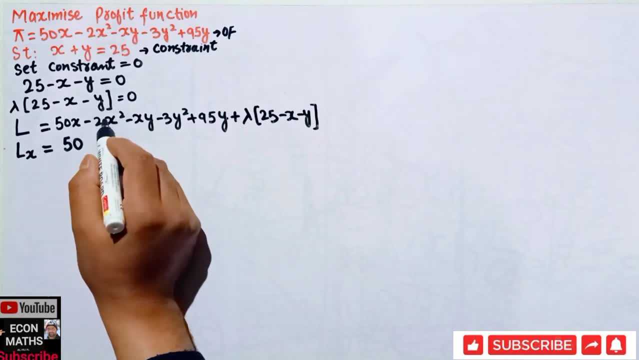 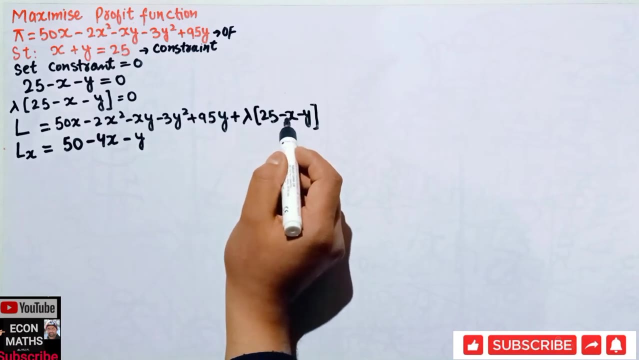 here this 2 will become coefficient. now two twos are four, that will become four x. now, two minus one is one minus y. here no x is involved. here no x is involved. here, uh, the coefficient, uh the derivative of x is one, so this will become minus lambda times one is minus lambda, so this is minus. 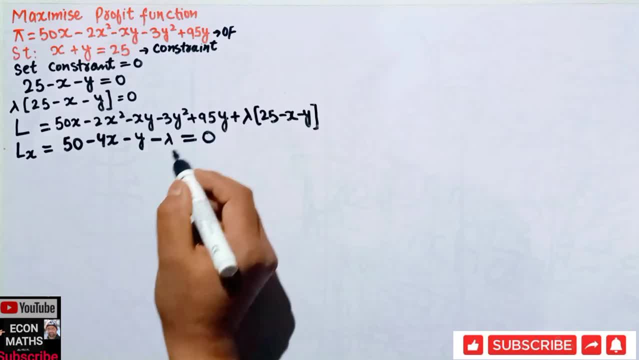 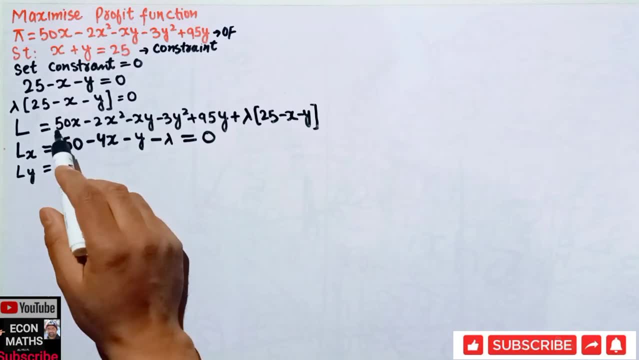 lambda and set it equal to zero. similarly we will with respect to y, partially. now, no y is involved here. no y is involved here. the derivative of y is one. so this will become minus x. so i will write here: it is minus x. here the derivative of y is: 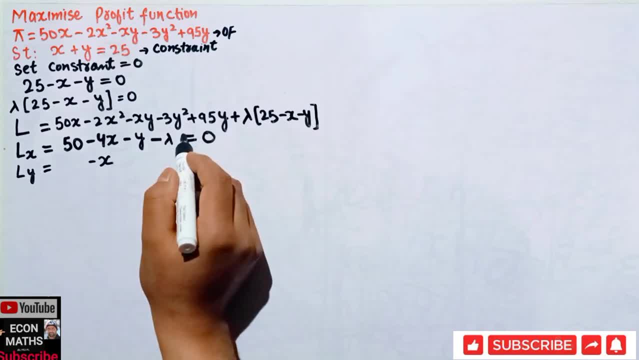 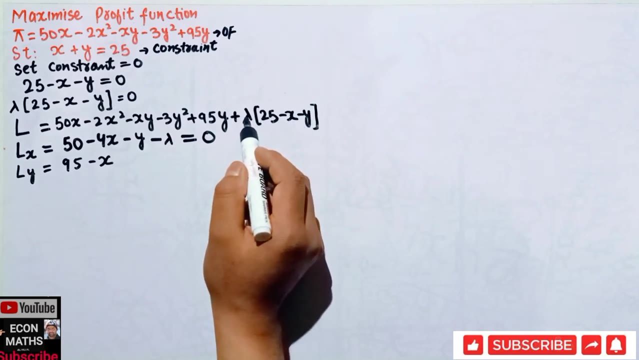 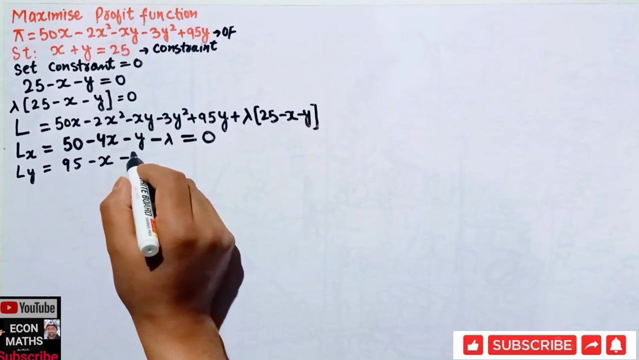 one. so this will become uh plus 95, so plus 95. so i will write it on this side. so we have 95 here. okay, so now we need to鉄 cop. our the derivative of y square is 0.. 0.. 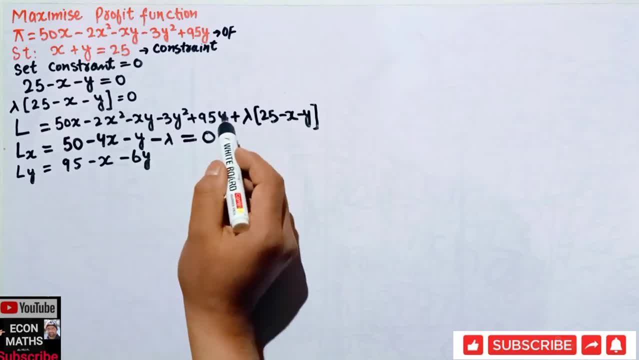 0.. 0.. 154, 154. y is 95, so i wrote it here. consistent with y is equal to 25 시간. i will write here negative and quarter minus 6, causing like this: that is what depends on the derivative of x, so this will become minus. 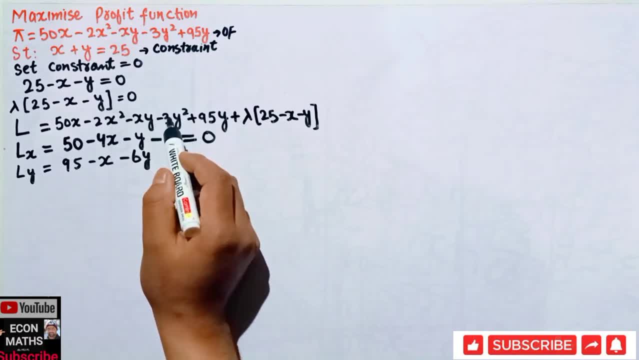 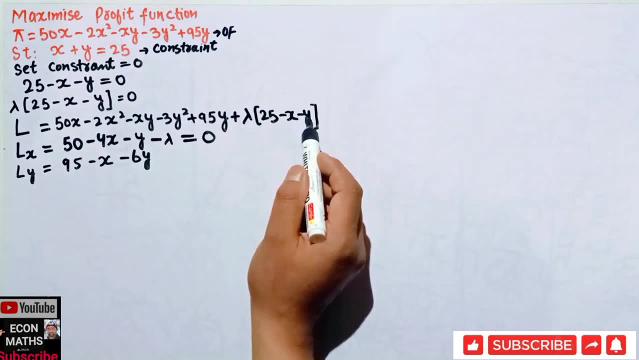 derivative of y square is 2y, so 3 into 2 is 6y. I write it on this side. similarly, here the derivative of y is 1, so this is minus 1 here. minus 1 into lambda is minus lambda, so I will write it here. 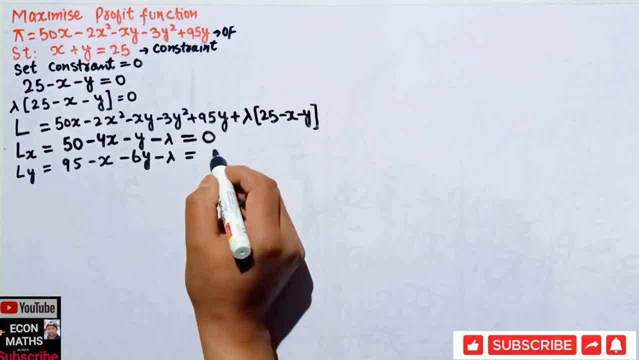 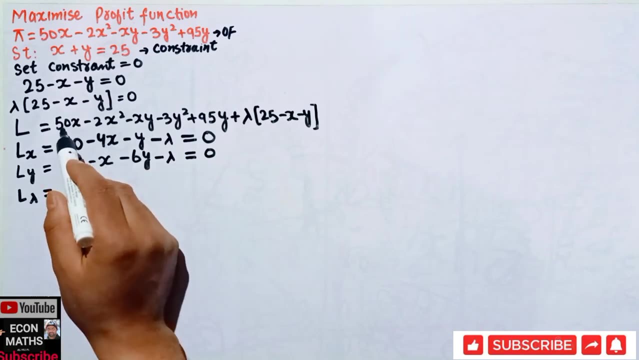 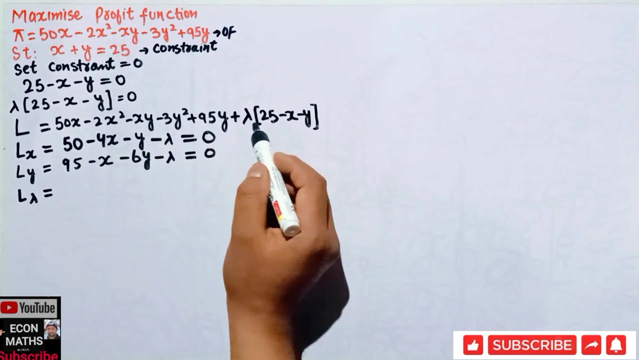 minus lambda and set it also equal to 0. okay, I hope I am making myself clear here. similarly, we will differentiate with respect to lambda. so we can see: in the first, first, second, third, fourth, fifth term there is no lambda involved. so there the derivative here is 0, here the derivative of: 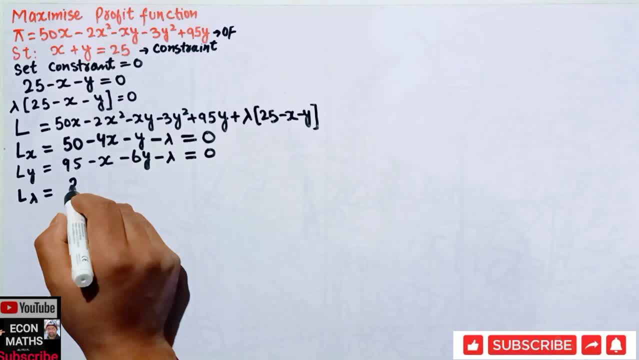 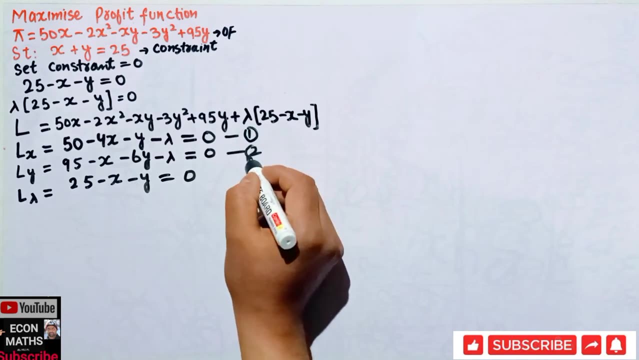 lambda is 1. so we are with this: 25 minus x, minus y is equal to 0. okay now, this is our first equation. let us say this is second equation. this is third equation. here we can see, we have the three variables. we have x, y and lambda. now how will we solve these very equations to get the optimal values of x? 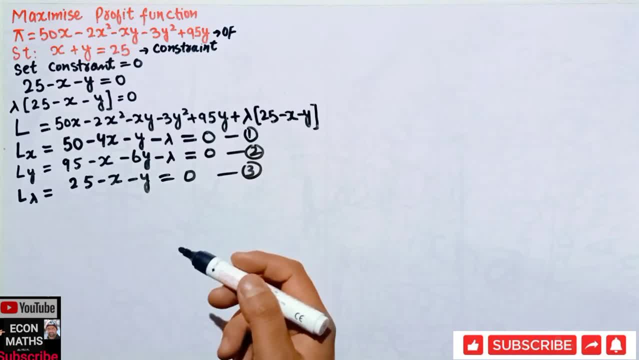 y and lambda. what will we do? first of all, we will eliminate this lambda. that means we will subtract the equation first by equation second. so I will write: equation one minus two will give us this will give us, this will give us- let us see here, 50 minus 90 for you. 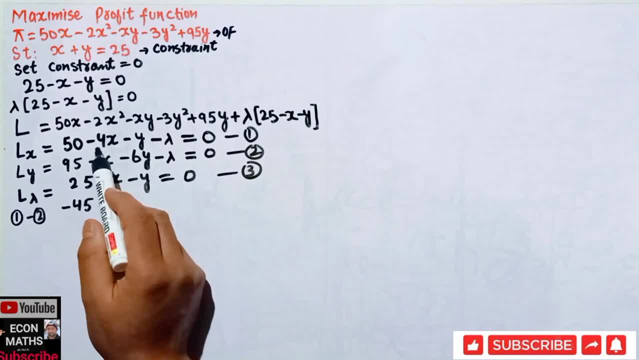 50 for us. so we will return 50 minus 90 for us, minus 45. okay now minus 4x, minus of the subtraction, so minus minus is plus. so this will give us this equation: 1 minus 90 for you, so minus 15.. minus 95, this is minus 45. okay now minus 4 x minus, ah, ah to subtraction. so minus, minus is plus. so this will give us equally plus. so minus, minus, minus is plus. so this will give us an ideal Danke in scientmaticieben. 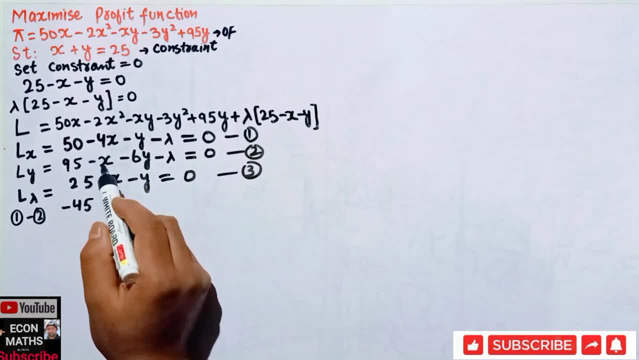 so this is minus 4x plus x. so this is minus 3x here. similarly, minus y, minus minus is plus here. so minus y plus x, y is plus 5y here. minus lambda, minus minus will become plus. so this is minus lambda, plus lambda will cancel each other. so we are with this equation. let this be equation 4. 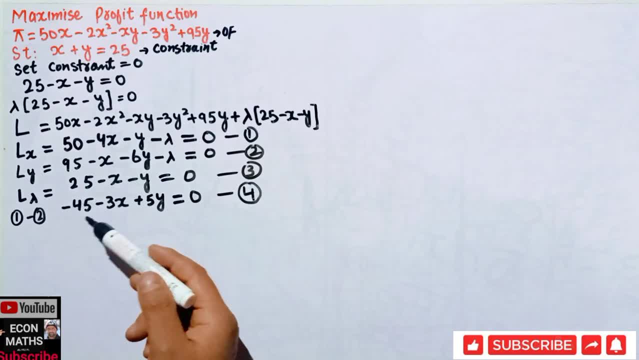 now we are only with the two variables. now, what will we do here? what will we do here to eliminate? we will multiply. first of all, here, it is to be seen, we have to make the coefficients in equation third and fourth the same of any variable. so we will make the coefficient of x same as in this. 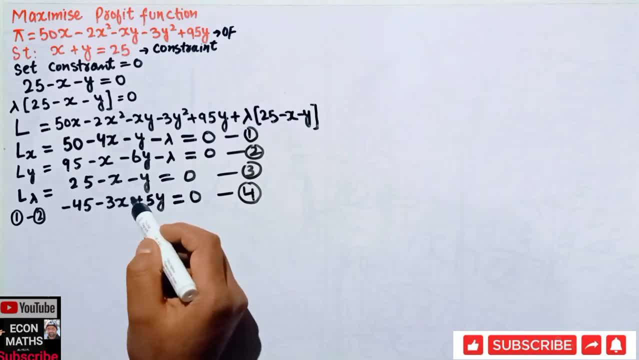 in the fourth equation. so for that we will multiply equation third by three, so multiplying equation third by three, so this will become 25 into 3. 25 into 3 is 75, so I will write it here: this is 75 minus 3x. minus 3y is equal to 0, and we will add, rather we will. 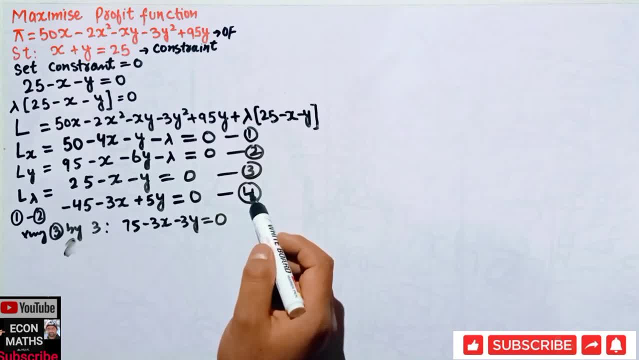 subtract equation 4 from this equation. so I will write here: this is minus 45. minus 3x plus 5y is equal to 0. it is to be here, sorry, it is to be remembered. here we are subtracting since. so this is minus 45 will become plus 45. this minus will. 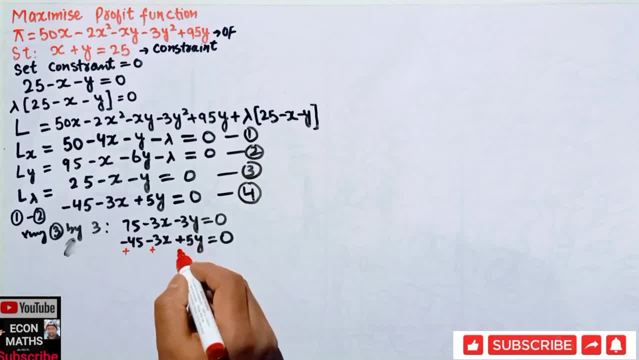 become plus. this plus 5 will become minus 5. so 75 plus 45 is 120. now minus 3x plus 3x. so this variable gets subtracted from this equation, so we will get canceled. here we are with minus 3y and minus 5i. this is minus. 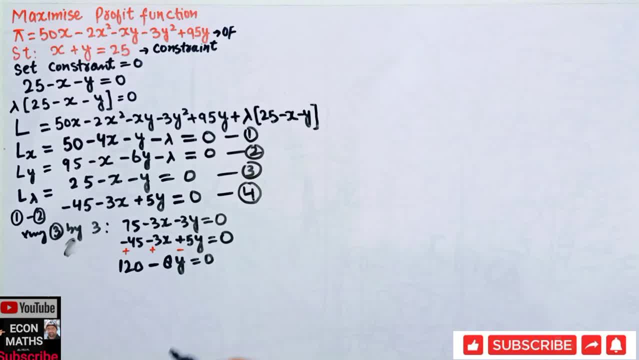 8y, which is equal to 0. now solving this will give us so this will become minus 8y is equal to transposing on RHS: this will become minus 120. now this minus minus gets cancelled. we are here with: y is equal to 120 divided by 8, which. 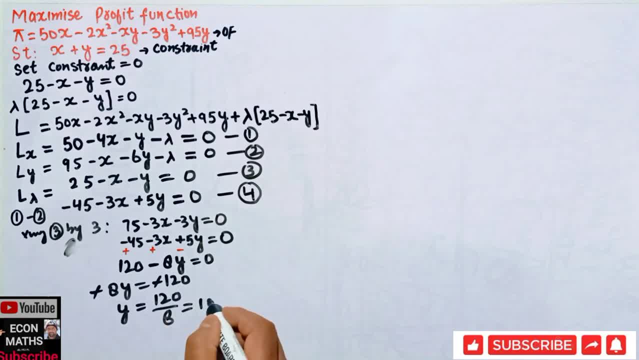 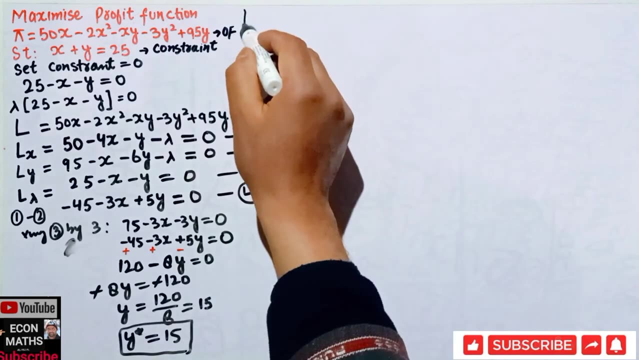 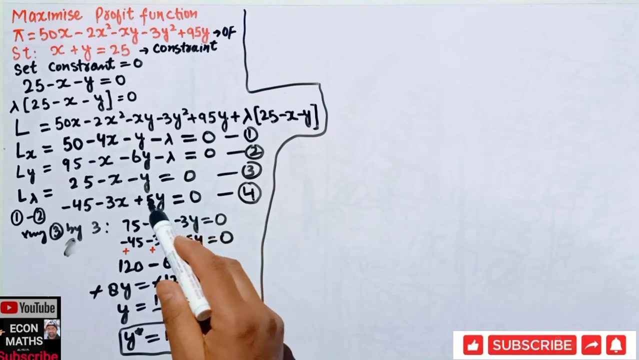 comes out to be 8. ones are 8, so 8. 5s are 40. so the optimal value of y is. so we got the value of y is equal to 15. okay, now we have to find the value of x. what will we do? we will put y is equal to 15 in equation third. so we will put: 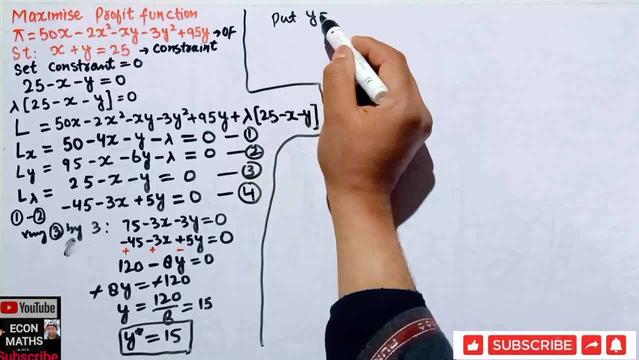 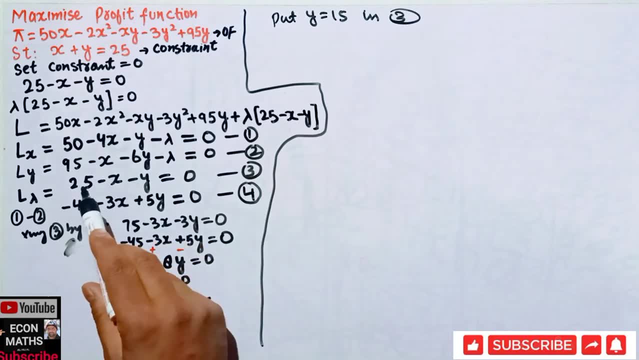 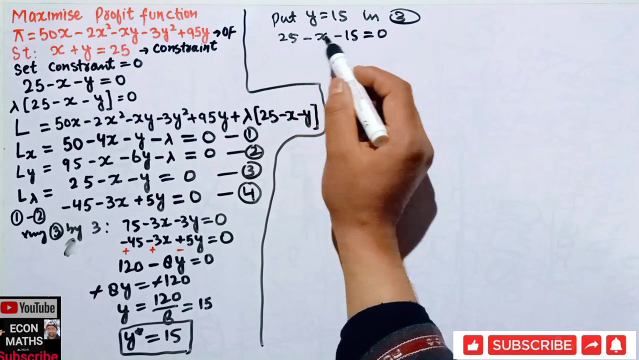 put, y is equal to 15, uh, in equation. third, so we have here 25, so i will write 25 minus x, minus the value of y, the value of y which we got, which is 15, which is equal to 0. now, 25 minus 15 is 10. so we have minus x minus 10. 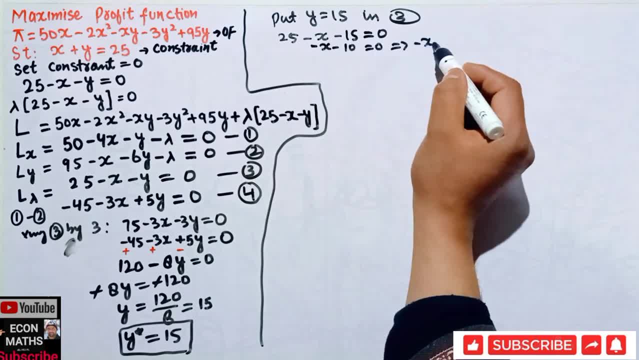 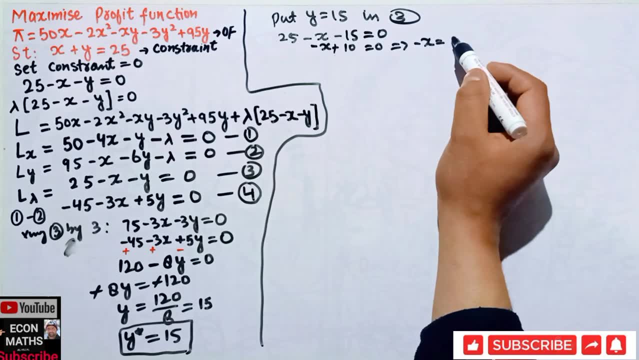 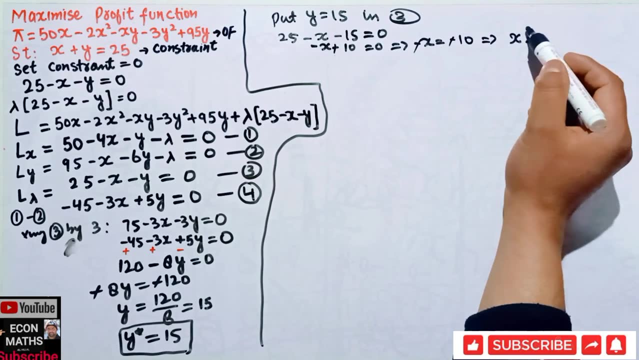 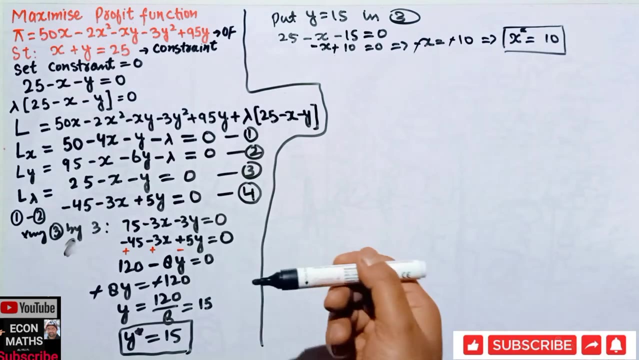 equal to 0 implies minus x is equal to sorry, this is plus 10, because 25 minus 15 is plus 10, so this will become minus 10 implies this minus minus gets cancelled. so the optimal value of x is 10. so we got the value of x and y. now we have to find the value of lambda, which 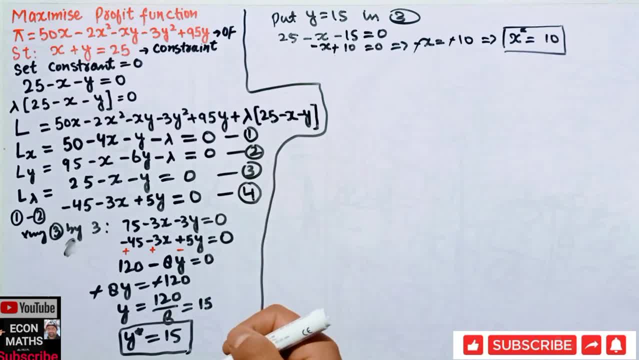 is very important in optimization process. now we have to find the value of lambda, which is very important in optimization process. now how will we find that very variable? we will put the value of x and y in either of the first two equations. let us say we put it in the equation first, so we will put put the value of x and y in. 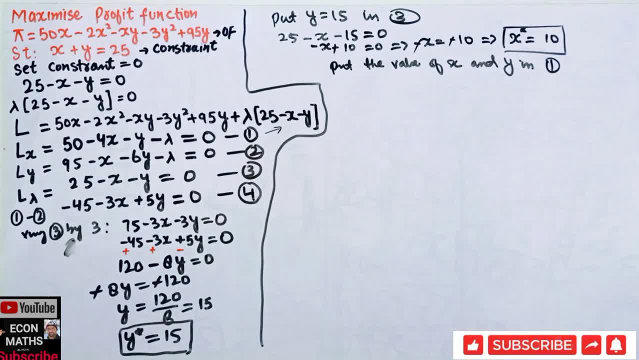 first in equation. first. now the first equation will look like: we have 50, 50 minus 4. the value of x is 10. so we will write 4 into 10. here minus y, the value of y is 15 minus lambda is equal to 0. solving this will become 50 minus 4. 10s are 40. 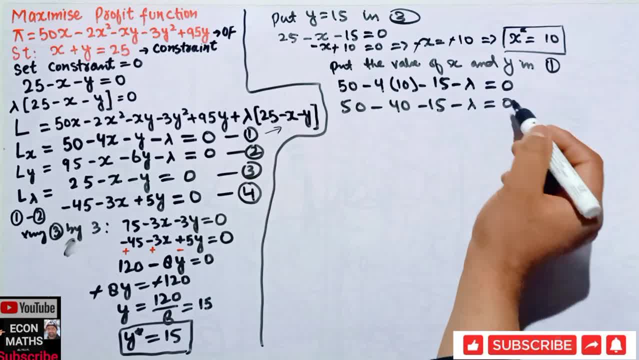 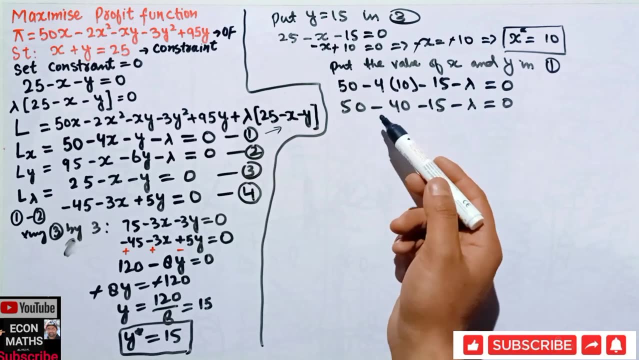 minus 15 minus lambda is equal to 0. now, 50 minus 40 is minus 10 and minus 10 and minus 15 is sorry, 15. 50 minus 40 is plus 10 plus 10 minus 15. so i will write here: 10 minus 15 is equal to 0. so this is minus 4: u minus lambda is equal. 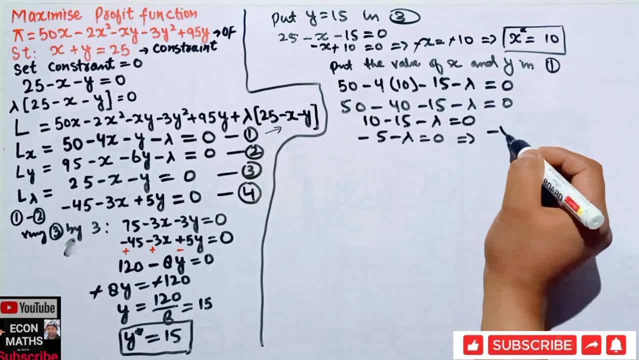 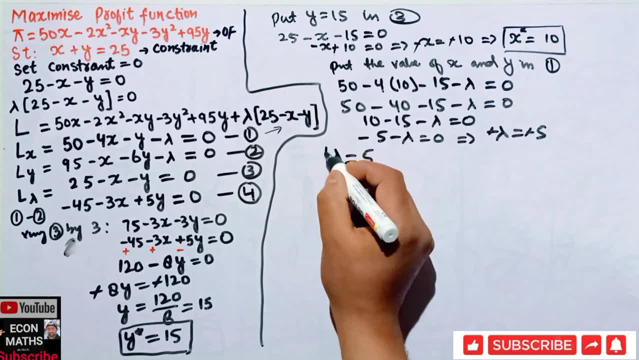 to 0 implies minus lambda is equal to minus 5. this lambda minus minus gets cancelled and we got the value of lambda is equal to 5. now this lambda has an important usage in the constrained optimization problem. this lambda shows as the marginal effector on the solution of the objective function when there is 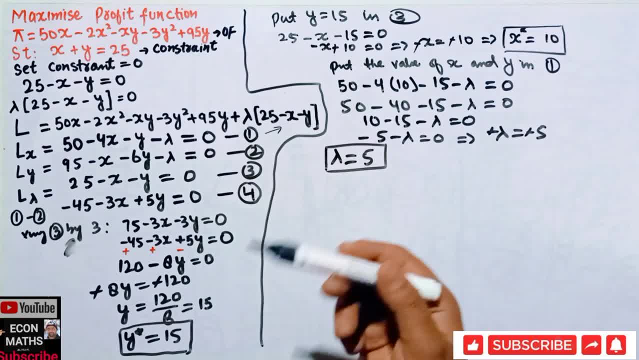 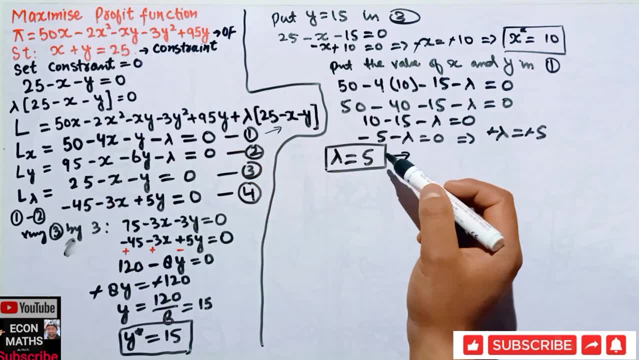 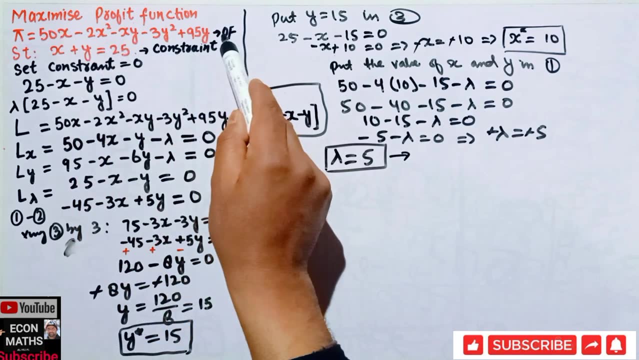 a unit change in the constant, that is, when there is unit change in the constant of the constant and this lambda shows, as the marginal effector on the objective function, that is how the profit will change, how the this profit function will change when there is change in the constant of the. 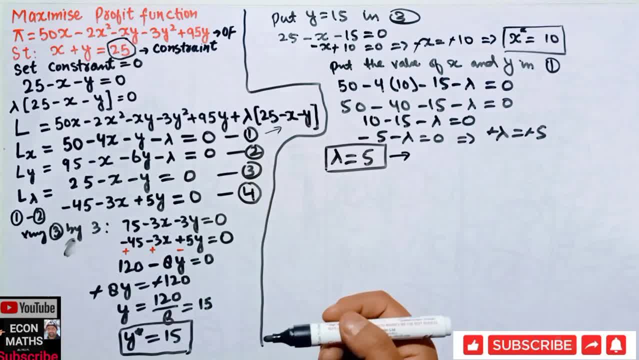 constrained. so let us, let us see: what does this mean? this mean is if change in total profit, that is, we can say if there is, if, if sorry, I will first write these, these two functions. so we have the profit function is 50 X minus true X square minus X, Y minus 3, Y square plus 95 Y and we have constant function. 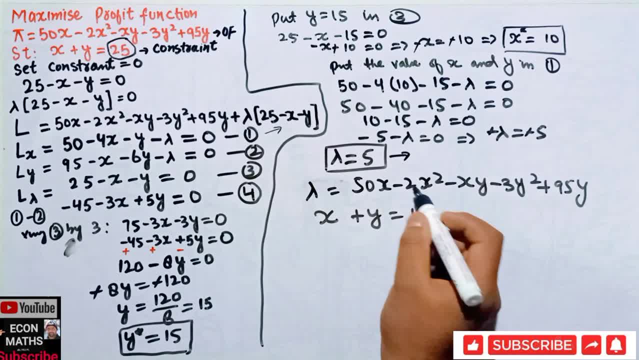 that is X plus Y is equal to 50. now we got the value of lambda is equal to 15. so here to make sure, this is pi. so this is our profit function. so we got the value of pi is equal to 15. sorry, pi is equal to 5. this pi is equal to 5 shows: